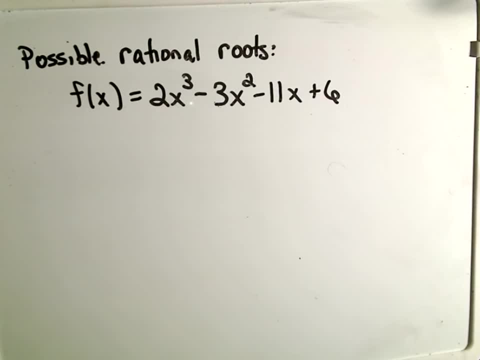 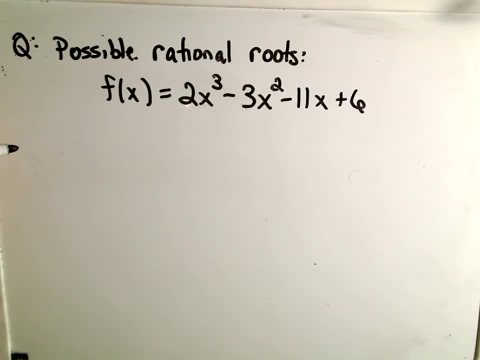 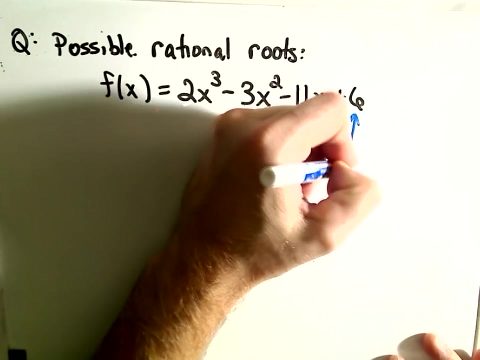 So I think it's best illustrated with an example. So the question is: what are the possible rational roots of this polynomial? 2x to the third, minus 3x squared, Minus 11x plus 6.. So again, basically, it says what you do is you look at the factors of the constant a sub 0,. 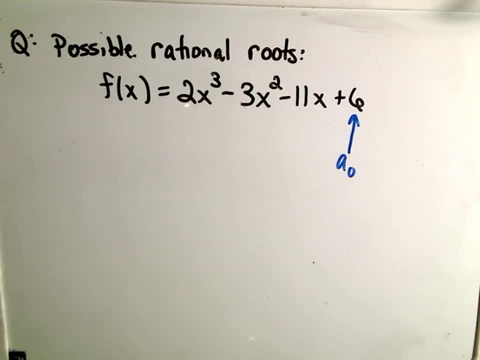 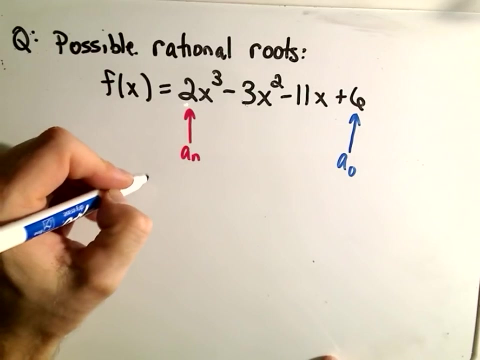 and then we look at factors of the leading coefficient. So that's our a sub n. You don't have to label them this way, but just to kind of correspond to what I had a second ago. If you think about factors of 6, well, factors of 6,. 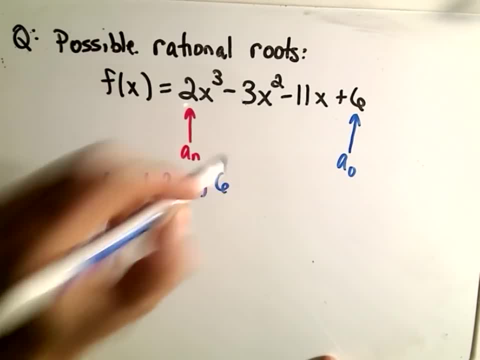 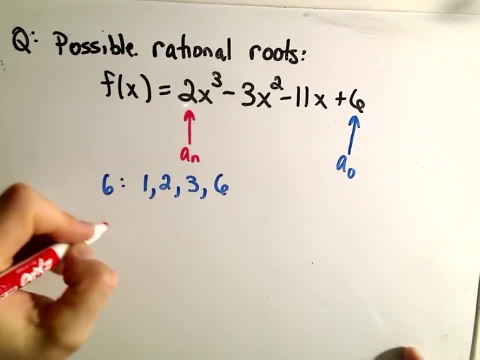 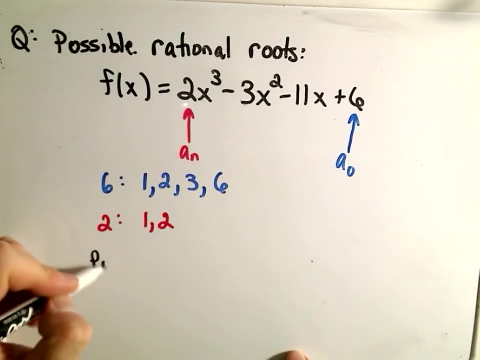 we have 1.. 2,, 3, and 6.. And then our factors of 2,. well, that's pretty easy. Our factors of 2 are just 1 and 2.. And now what we do? it says the possible rational roots. 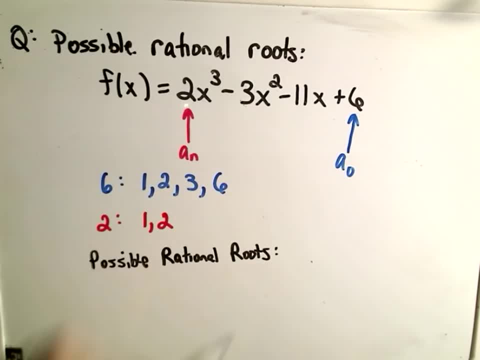 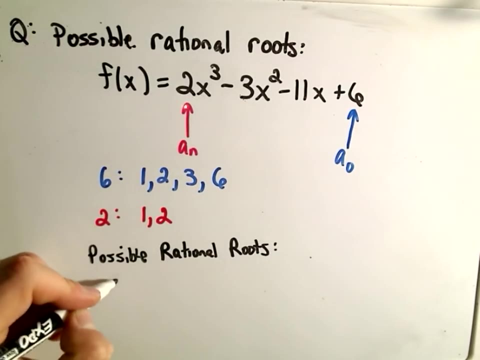 And remember, a rational number is just a number that can be written as a decimal. It's a number whose either the decimal terminates or the decimal has a repeating pattern to it. That's a rational number. It says the possible rational roots. basically it says you take all possible combinations of the numbers here on the top. 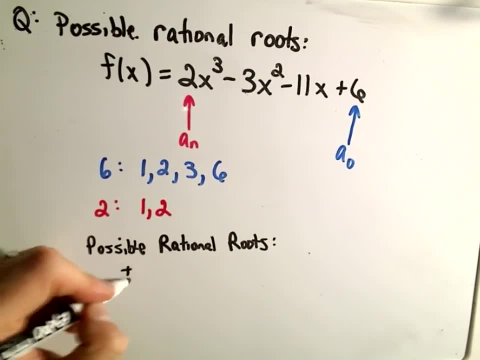 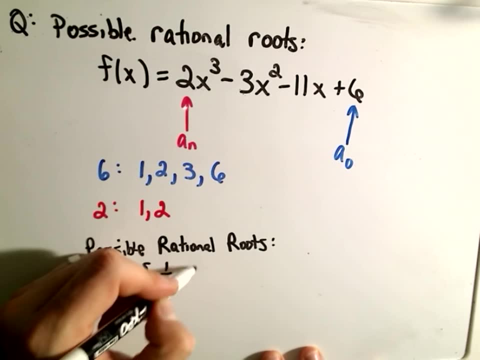 divided by numbers on the bottom. So I'm going to write them all out and then just get rid of duplicates. So it says you would get positive- negative 1 over 1, positive negative 1 over 2 would be a candidate: positive, negative 2 over 1,. 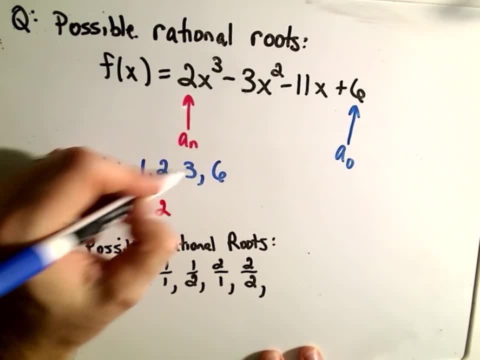 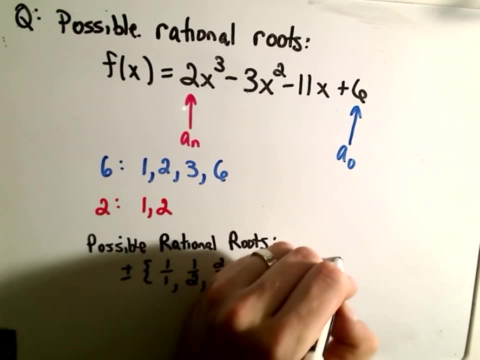 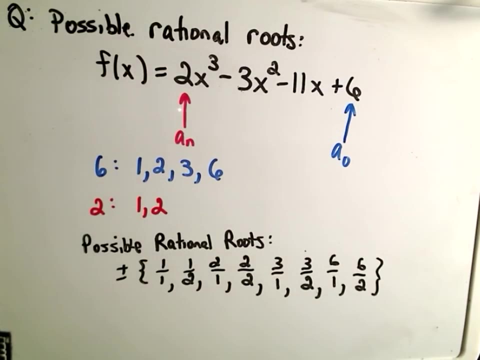 positive negative 2 over 2, positive negative 3 over 1, positive negative 3 over 2, positive negative 6 over 1, positive negative 6 over 2.. Okay, these are all the possible rational roots for this polynomial. 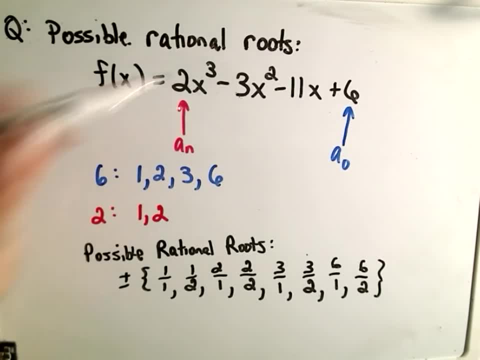 And again, remember, a root is just a number, that if we plug it in for x, we'll get 0 out at the end. So let's see what we have. We have 1 over 1, which is 1.. 1 over 2,, which is a half. 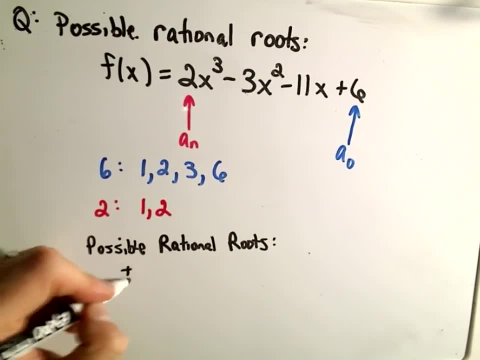 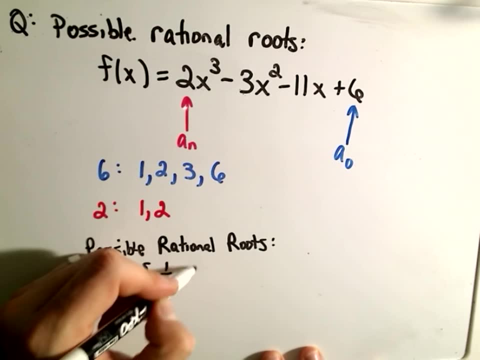 divided by numbers on the bottom. So I'm going to write them all out and then just get rid of duplicates. So it says you would get positive- negative 1 over 1, positive negative 1 over 2 would be a candidate: positive, negative 2 over 1,. 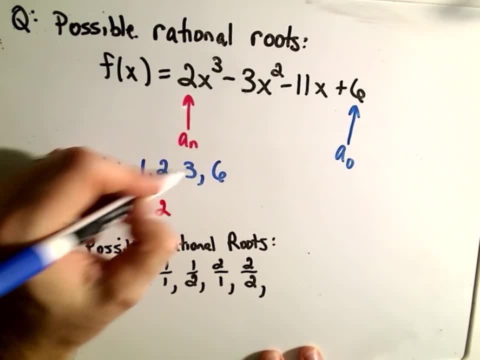 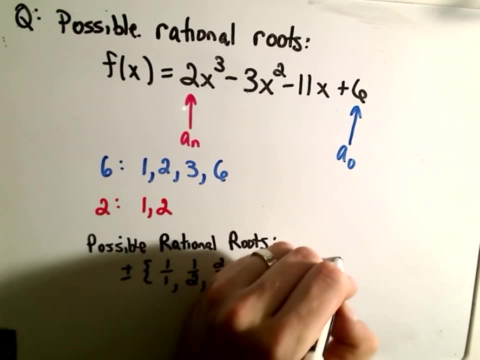 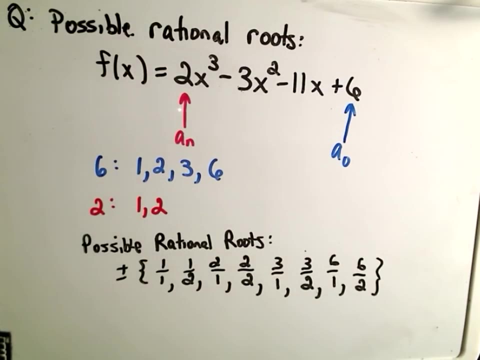 positive negative 2 over 2, positive negative 3 over 1, positive negative 3 over 2, positive negative 6 over 1, positive negative 6 over 2.. Okay, these are all the possible rational roots for this polynomial. 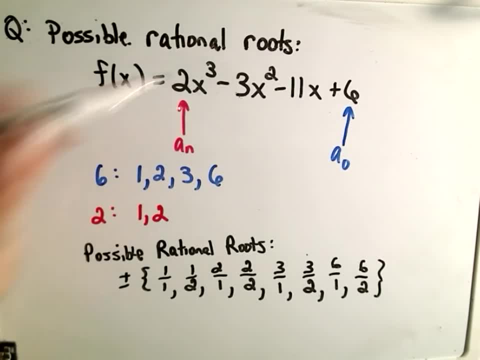 And again, remember, a root is just a number, that if we plug it in for x, we'll get 0 out at the end. So let's see what we have. We have 1 over 1, which is 1.. 1 over 2,, which is a half. 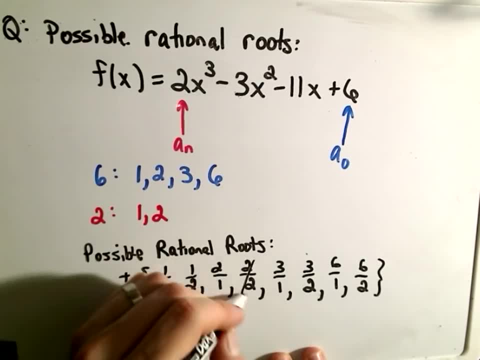 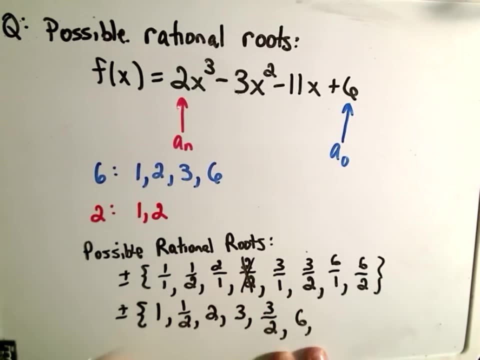 2 over 1 is 2.. 2 over 2 is 1, so we already have that. 3 over 1 is 3.. We have 3 halves, We have 6.. And again, 6 over 2 is 3, so we already have that one listed as well. 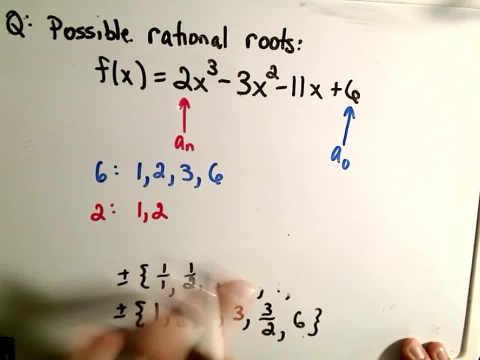 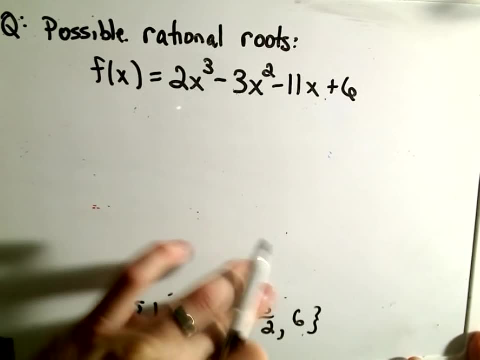 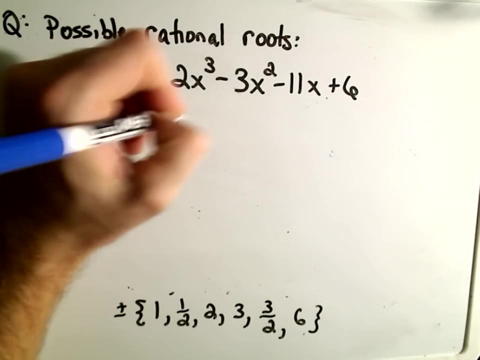 Excuse me. So these are our possible rational roots And let's just check and see. maybe we can figure out what the roots of this polynomial are. So the question could be: is x equals 1 a root? So let's see if x equals 1 is a root. 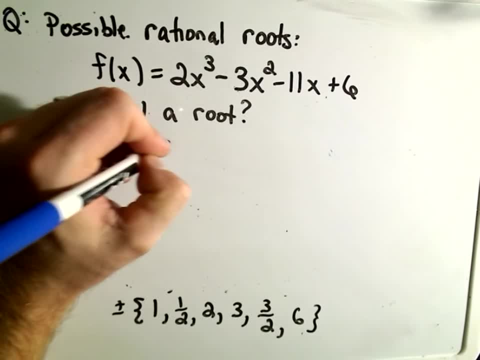 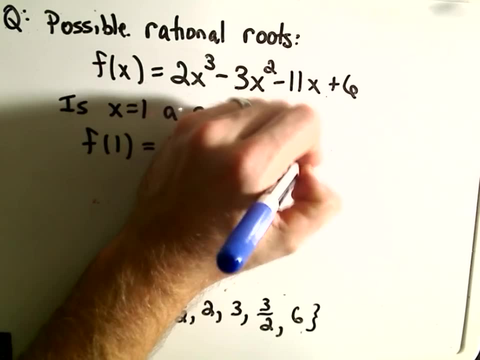 So that means if we plug 1 in, we'll get 2 times 1 cubed, minus 3 times 1 squared, minus 11 times 1, plus 6.. And the question is: does this equal 0?? 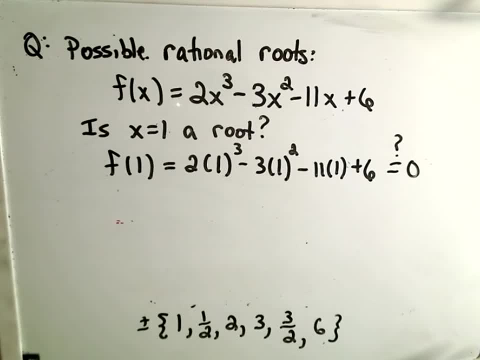 That's what it means to be a root. So all we have to do is just simplify this down. Well, 1 cubed is 1, times 2 is 2.. 1 squared is 1, times 3 is 3,. 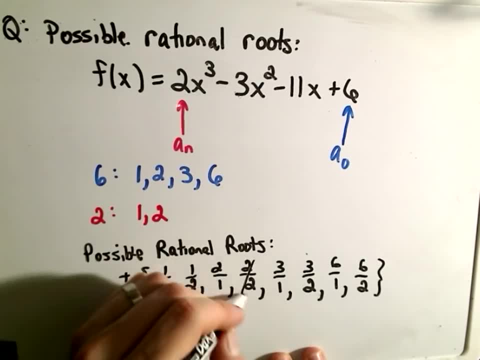 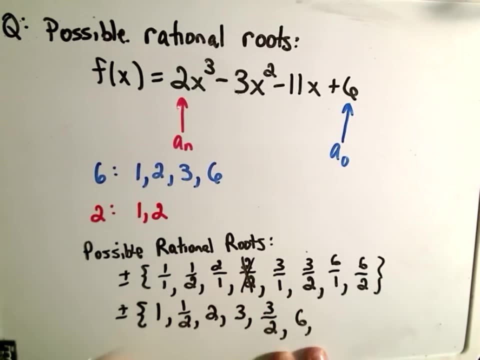 2 over 1 is 2.. 2 over 2 is 1, so we already have that. 3 over 1 is 3.. We have 3 halves, We have 6.. And again, 6 over 2 is 3, so we already have that one listed as well. 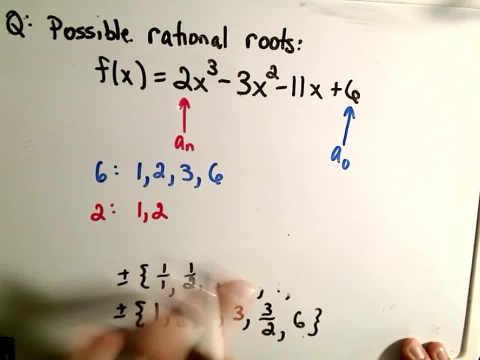 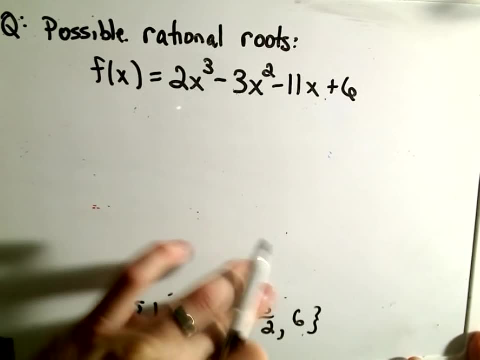 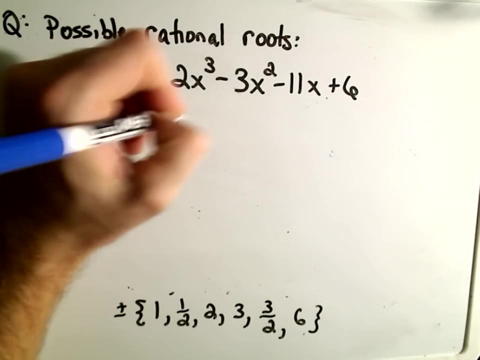 Excuse me. So these are our possible rational roots And let's just check and see. maybe we can figure out what the roots of this polynomial are. So the question could be: is x equals 1 a root? So let's see if x equals 1 is a root. 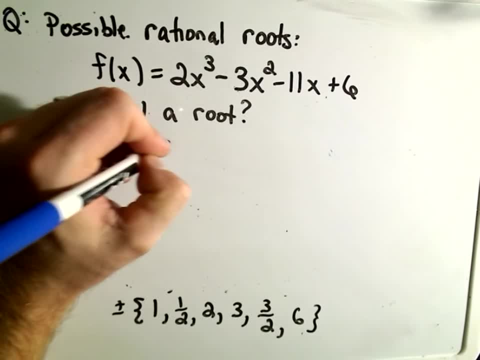 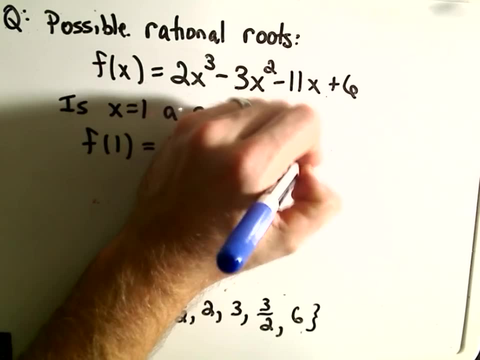 So that means if we plug 1 in, we'll get 2 times 1 cubed, minus 3 times 1 squared, minus 11 times 1, plus 6.. And the question is: does this equal 0?? 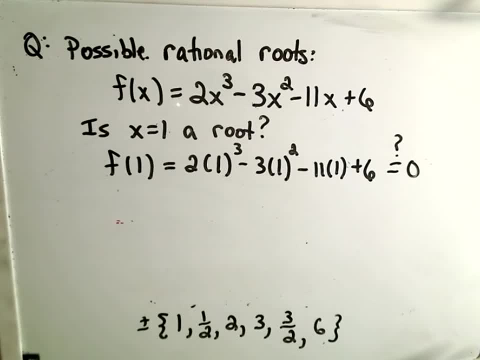 That's what it means to be a root. So all we have to do is just simplify this down. Well, 1 cubed is 1, times 2 is 2.. 1 squared is 1, times 3 is 3,. 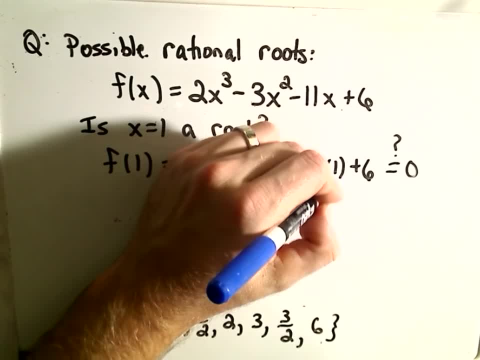 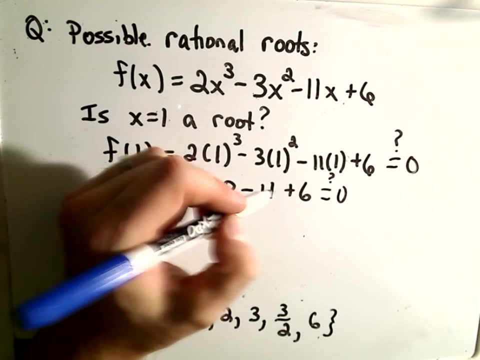 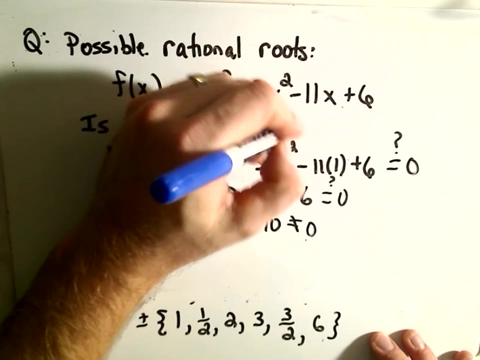 minus 11, plus 6.. Does that equal 0?? Looks like we get negative 5 minus 11,, which is negative 16, plus 6 is negative 10.. Well, that certainly doesn't equal 0. Which means no x equals 1 is not a root. 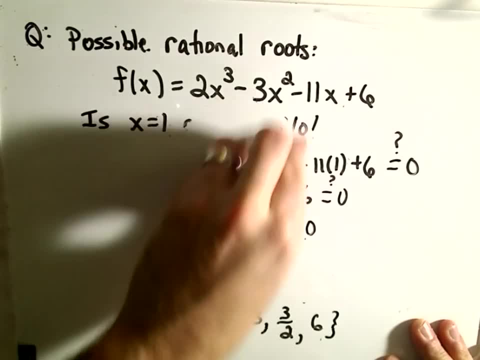 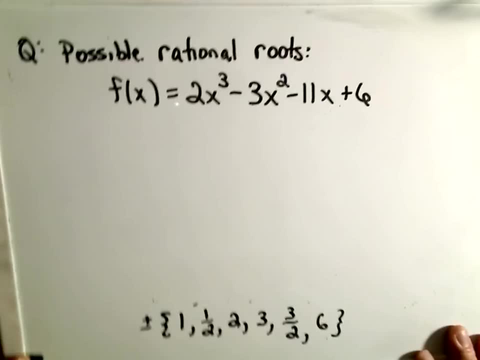 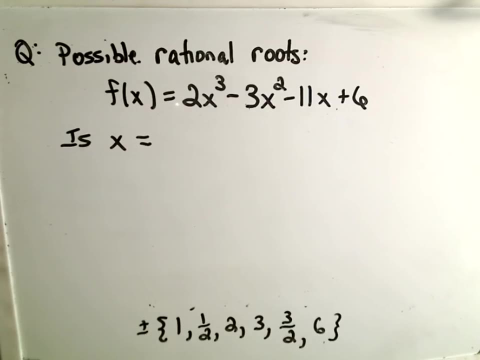 Okay, so let's check one more and then I'll tell you the solutions and you can check them out here, because I won't have time to check them all. It'll get kind of tedious. So maybe we can check. is x equals? 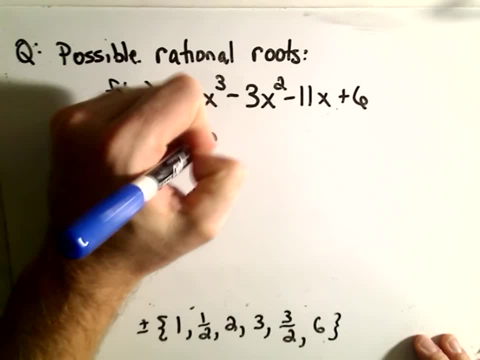 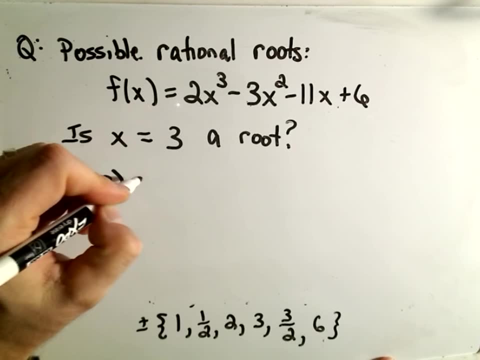 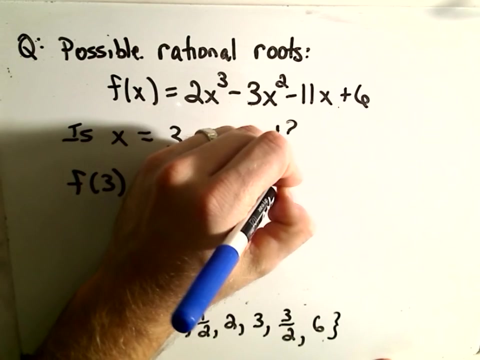 how about positive 3 a root? Well, let's check and see. So if we plug 3 in, it says f of 3 is 2 times 3, cubed minus 3 times 3, squared minus 11 times 3,. 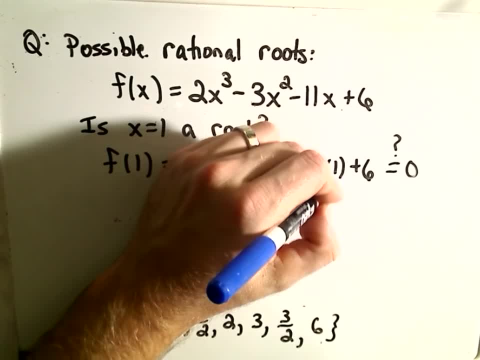 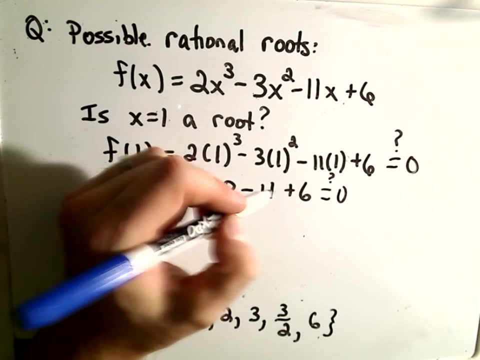 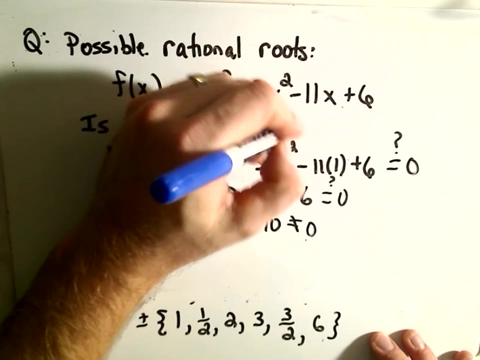 minus 11, plus 6.. Does that equal 0?? Looks like we get negative 5 minus 11,, which is negative 16, plus 6 is negative 10.. Well, that certainly doesn't equal 0. Which means no x equals 1 is not a root. 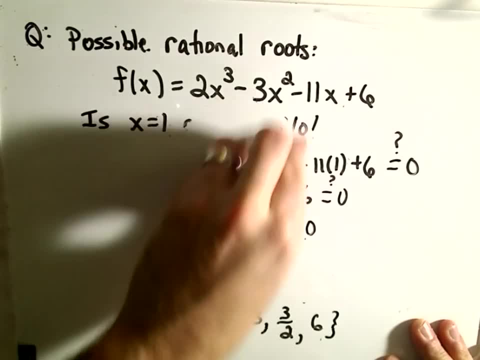 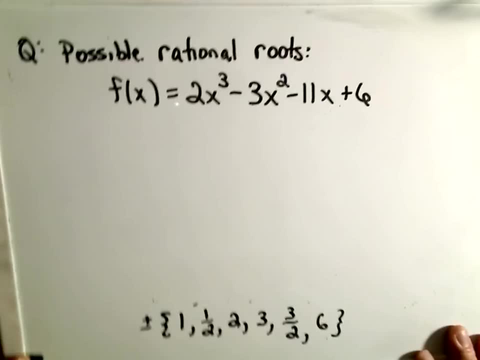 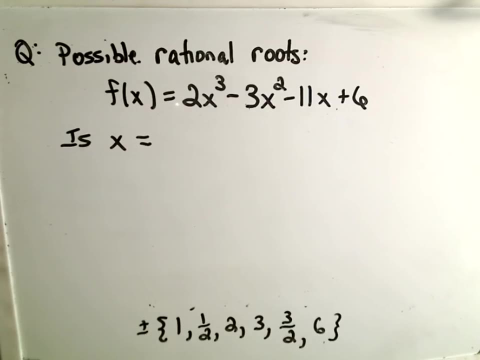 Okay, so let's check one more and then I'll tell you the solutions and you can check them out here, because I won't have time to check them all. It'll get kind of tedious. So maybe we can check. is x equals? 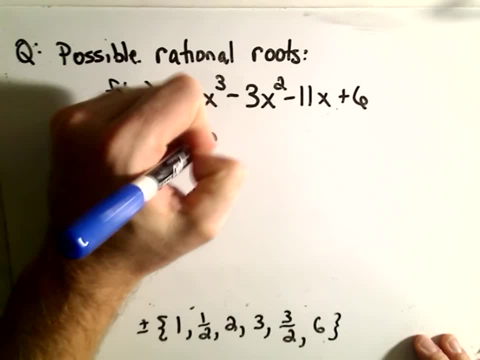 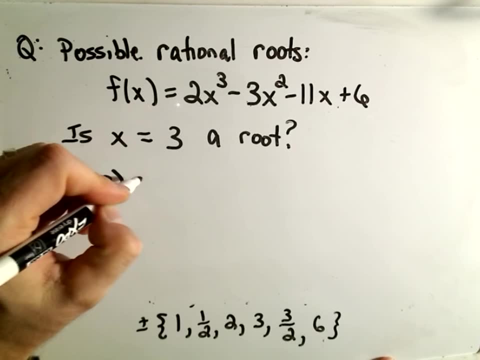 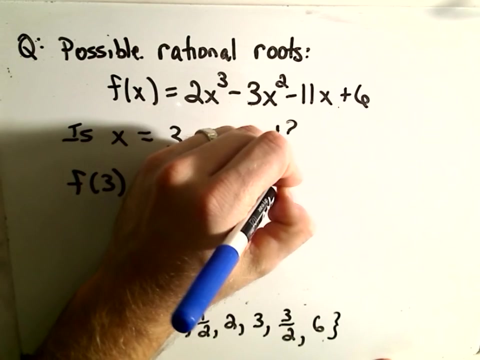 how about positive 3 a root? Well, let's check and see. So if we plug 3 in, it says f of 3 is 2 times 3, cubed minus 3 times 3, squared minus 11 times 3,. 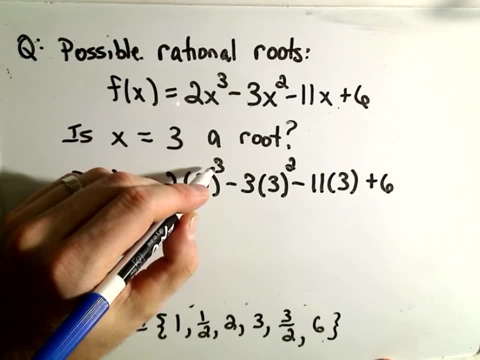 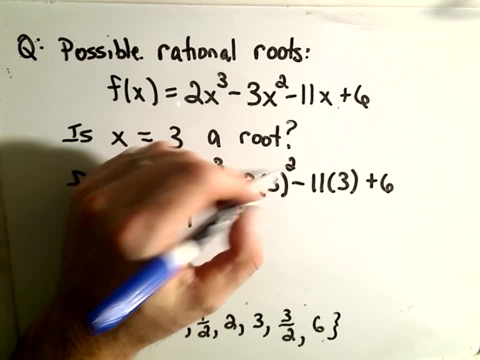 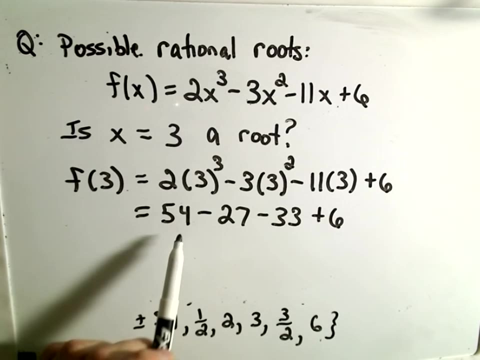 plus 6.. 3 cubed is 27.. 27 times 2 is 54.. 3 squared is 9.. 9 times 3 is 27, minus 33, plus 6.. Okay, 54 minus 27,. 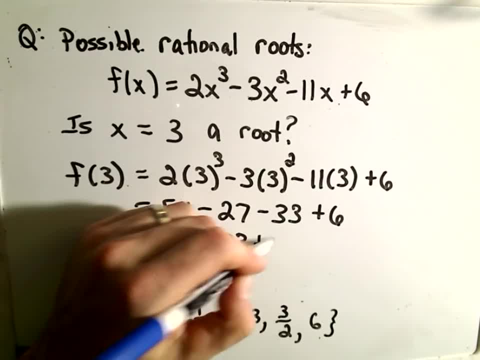 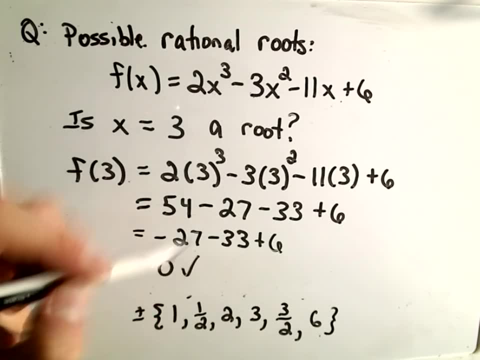 that's negative 27, minus 33 plus 6.. Well, negative 27 minus 33 is negative 6.. Negative 6 plus 6 is 0.. So yes, 3 is a root in this case And you can actually check. 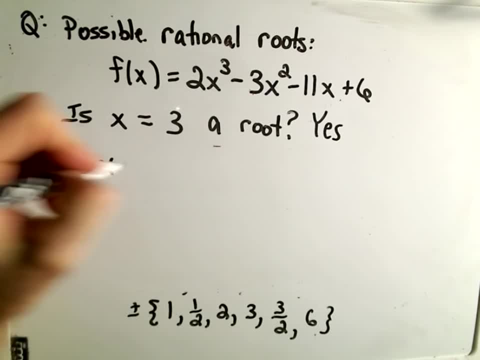 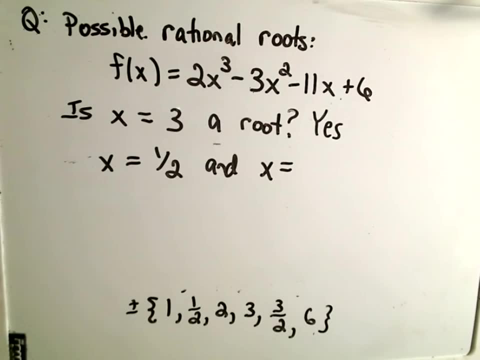 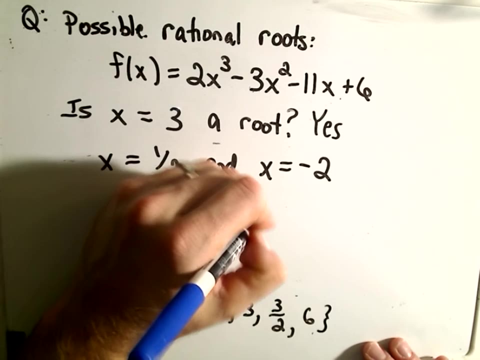 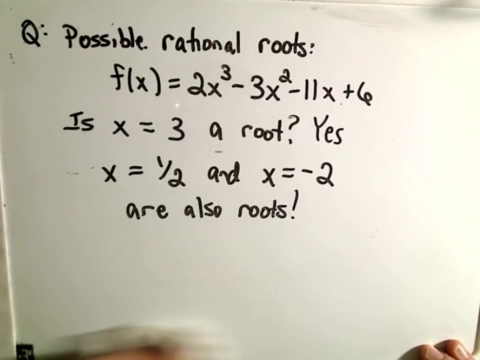 I think my arithmetic was okay here: x equals 1 half and x equals negative. 2 are also roots Okay. so in this case my polynomial I set it up to actually have 3 rational roots. But again, that doesn't have to happen at all. 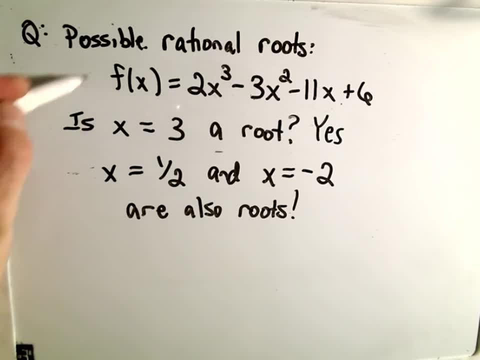 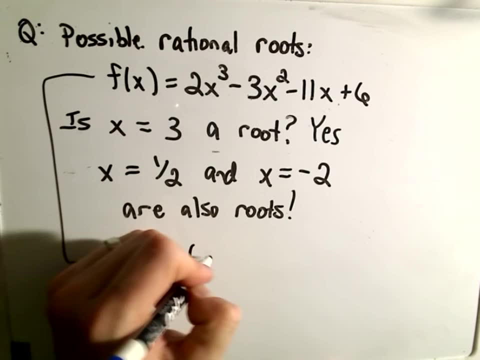 Well, one last question: If we know the roots, how does this polynomial factor? Well, if we know the roots, we can factor it as well. you just take the opposite sign. basically, So x minus 1 half is a factor.